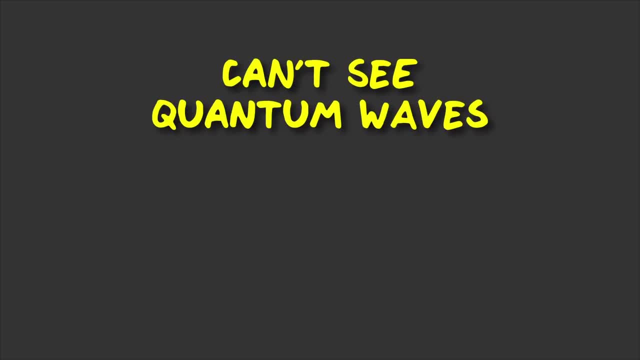 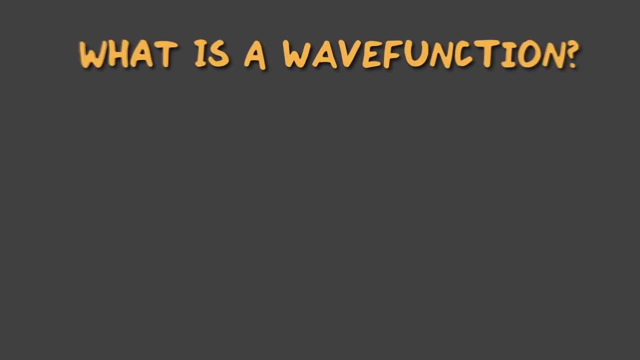 on that subject. But even though we'll never be able to see a quantum wave function, we can do the next best thing and visualise the mathematical equations. So this is what the maths says the wave function looks like. These two are mathematically equivalent, although this one's easier to do calculations with. 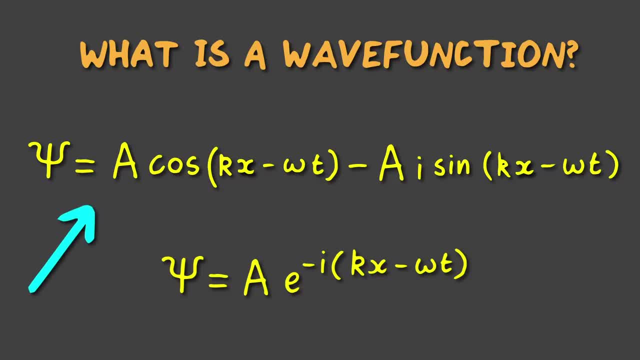 but we'll use this form for this video as it's easier to visualise. This wave function depends on time and one dimension of space, which is a simplification from a real particle which exists in three dimensions of space. but this simplification allows us to plot this function, So let's do that. 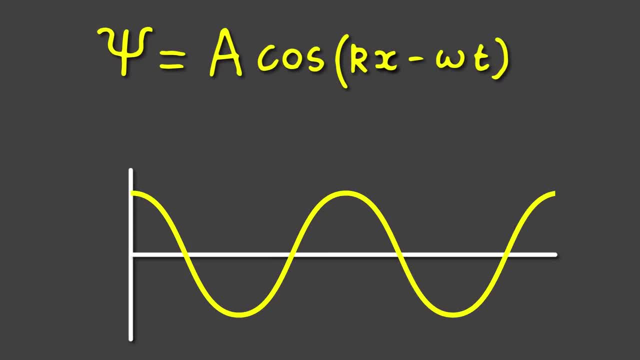 We'll just plot the first part of this wave function. to begin with, This is simply a cosine wave. Note that the k is a variable controlling the size of the wavelength, the omega controls the oscillation frequency and the prefactor a controls the amplitude. So different parameters. 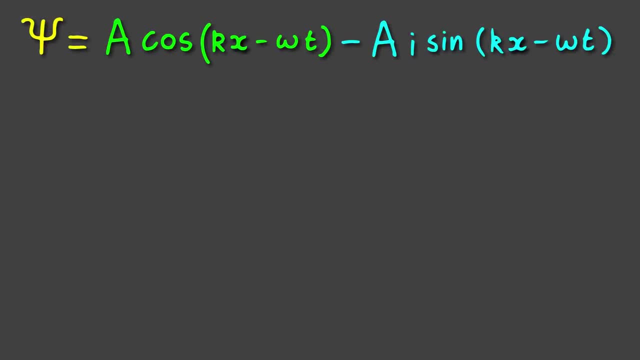 will make different waves. Now, to plot the second part of the wave, we're going to need another axis, even though the wave is one dimensional. This is because the sine part of the wave function is multiplied by the imaginary number, i making it a complex wave function. 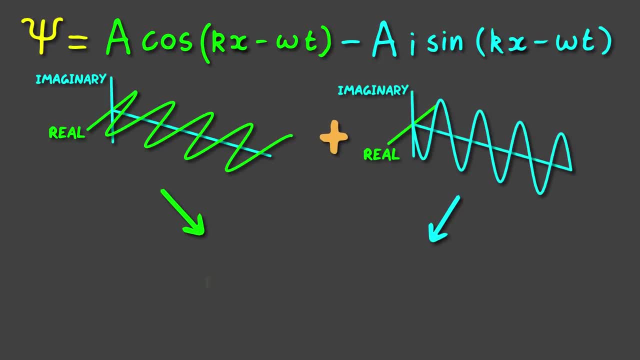 So here they are, both plotted independently. But if we plot the whole thing together we get this: a spiral of complex values which would go from minus infinity to plus infinity. but I'm just plotting a section of it here. This is fixed at one point in time, but if we turn time on we get an oscillation which 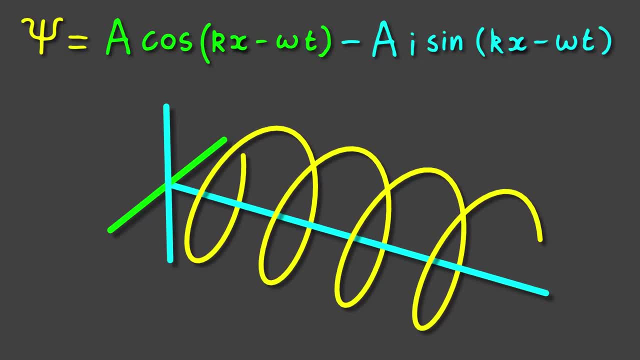 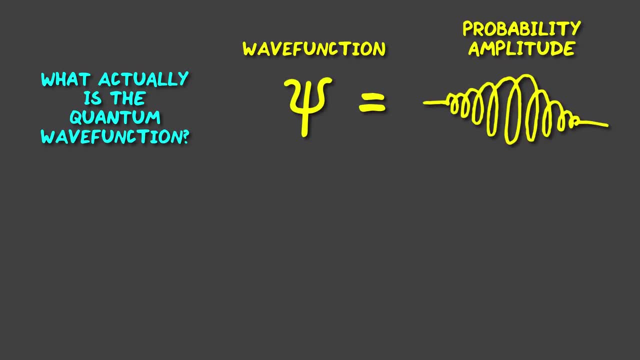 in this case manifests as a winding of the spiral. So that's what a quantum wave function looks like. But what actually is it? It's called a probability amplitude and isn't anything physical on its own. but if you take the mod, 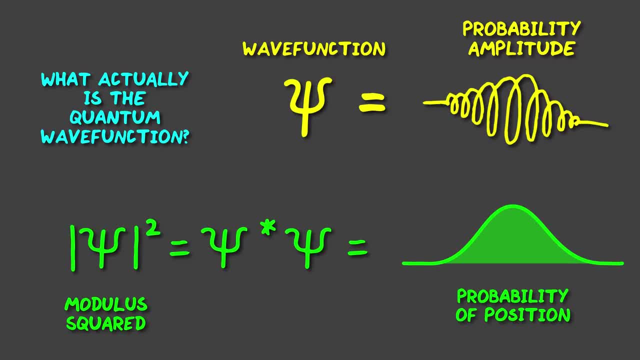 squared of the amplitude. it tells you the probability of finding the particle at any point in this one dimensional space. So we can extract the position of a particle from this wave function. Actually, the wave function doesn't just tell you about the probability of position, but all other measurable. 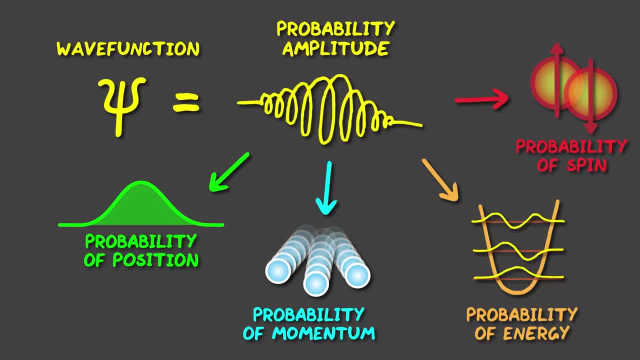 physical quantities like momentum or energy or spin. We just need to do different mathematical operations on the wave function for each one. But overall the wave function is a mathematical tool which keeps track of all of the properties of a quantum particle and explains our observations of the probabilistic nature of where particles 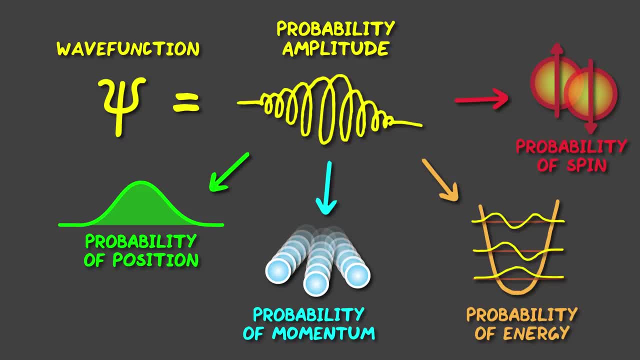 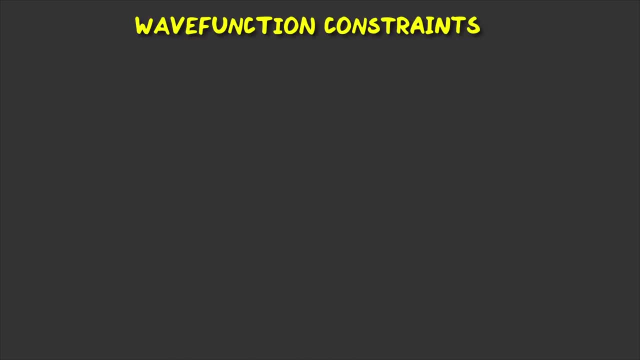 appear when we do experiments on them. So far, I've given you one example of a wave function, but there are many other possibilities. They just have to satisfy a set of constraints, which I'll be drawing on one axis for clarity. Firstly, a wave function must be a solution of the Schrodinger equation which I mentioned. 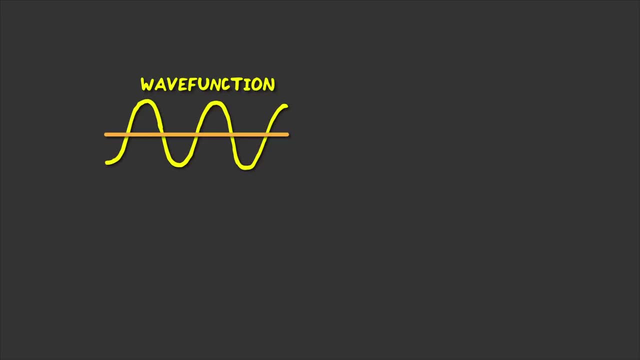 at the beginning. Secondly, when you calculate a probability from the wave function, you'll get a probability distribution And the area of this needs to equal one, because there has to be a definite probability. you'll find the particle somewhere. This means that the 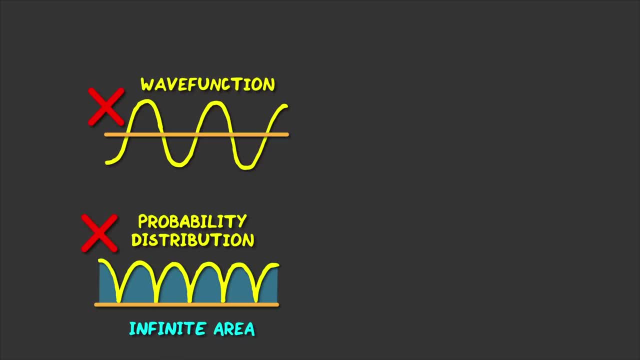 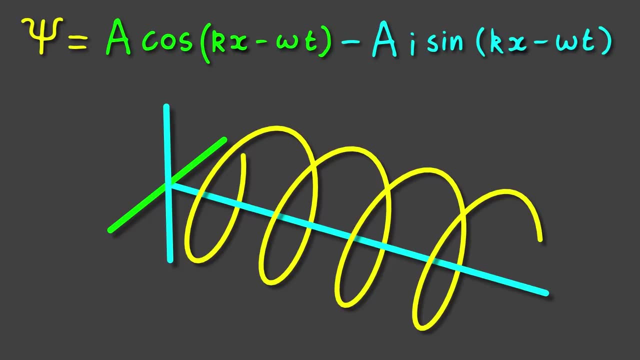 original wave function can't have an infinite area underneath it. Technically we say that the wave function must be normalisable. So my visualisation from earlier is not the same as the original wave function, but it's a little bit different. It's not actually allowed- because it goes from minus infinity to plus infinity- To be. 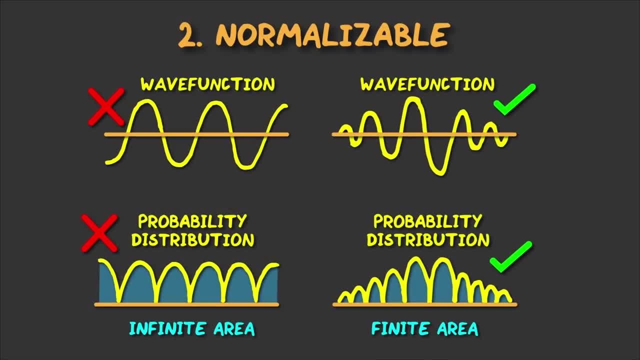 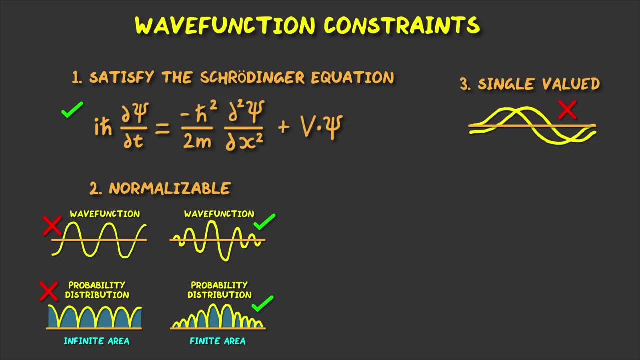 valid, it would have to go to zero, as x goes to infinity. Thirdly, the wave function must be single-valued. Also, it must be continuous, so have no breaks in it. And the slope of the wave function must be continuous, so no discontinuities in the gradient. 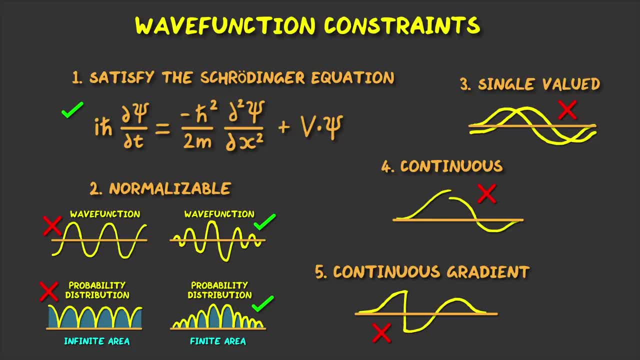 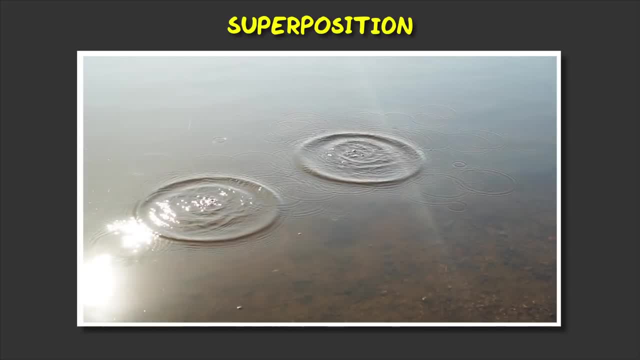 like this. So those are the conditions quantum wave functions have to meet. Finally, let's look at superposition. This is a property that's also not unique to quantum mechanics. If you have two sets of ripples and water that overlap any point. 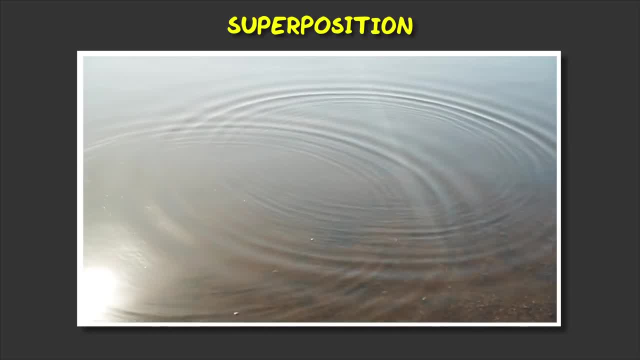 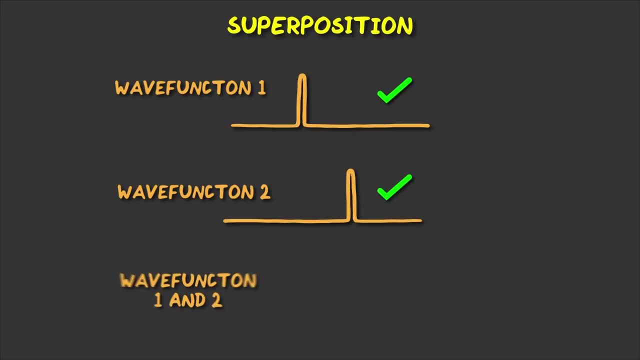 will feel the two waves added together and this is a superposition of waves In quantum mechanics. if you have two or more wave functions that are valid solutions of the Schrodinger equation, then any combination of these wave functions is also a valid solution. 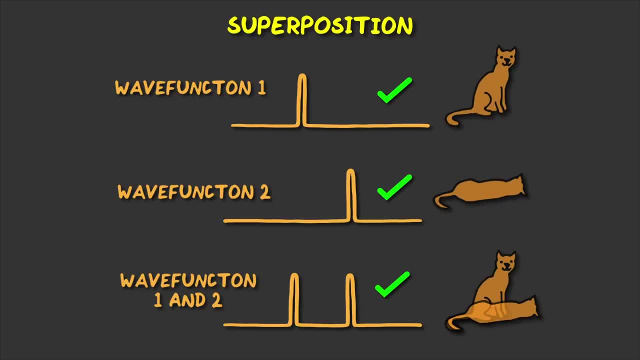 And this is where the idea comes from- that Schrodinger's cat can be dead and alive at the same time. Although there's no doubt about that, There's no doubt about that This never actually happens because of other quantum phenomena: entanglement and decoherence. 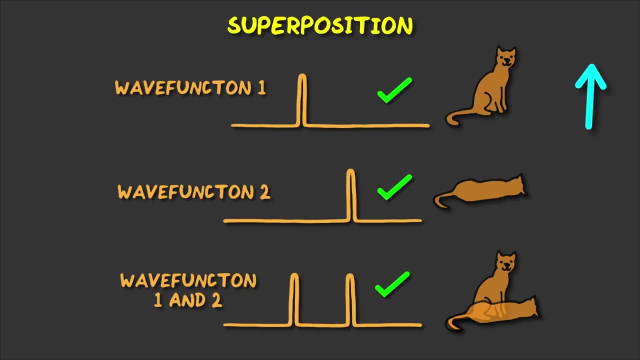 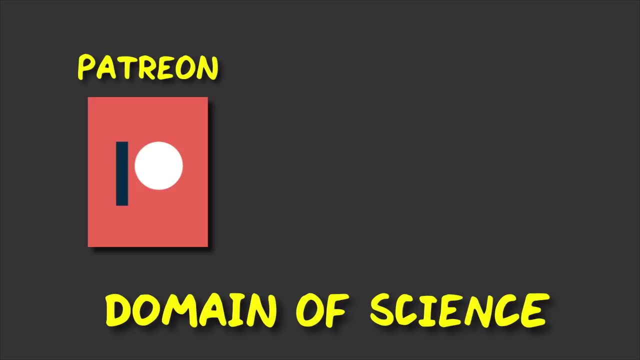 These are beyond the scope of this video, but here's an excellent video on the subject from Sabine Hossenfelder for those of you who'd like to delve deeper. This video was made possible thanks to the kind support of my patrons on Patreon and.